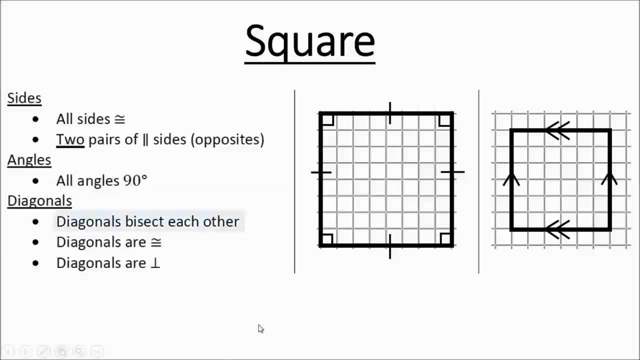 Next we're going to talk about diagonals. Diagonals bisect each other. That means they cut each other in half. Also, these diagonals are congruent, So two things here. We've got the entire diagonal being the exact same measurement as the other diagonal. 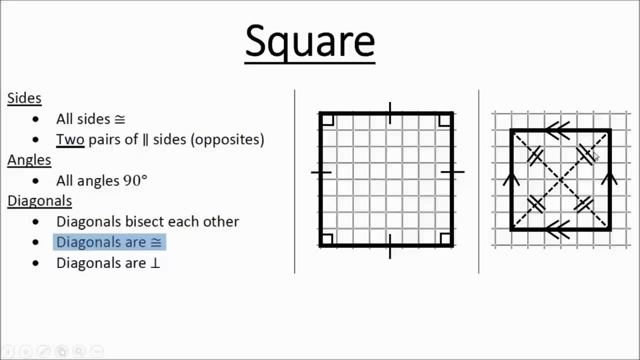 And then the way these are marked. that means that they are chopped in half, So this half is equal to this half, and so on. Also, the diagonals are perpendicular, So you'll see these two diagonals meet And you'll see a 90 degree mark there. 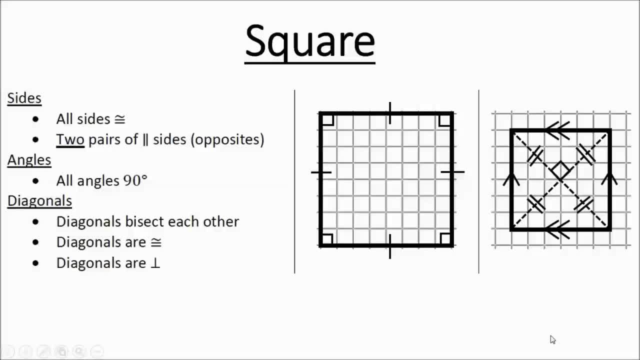 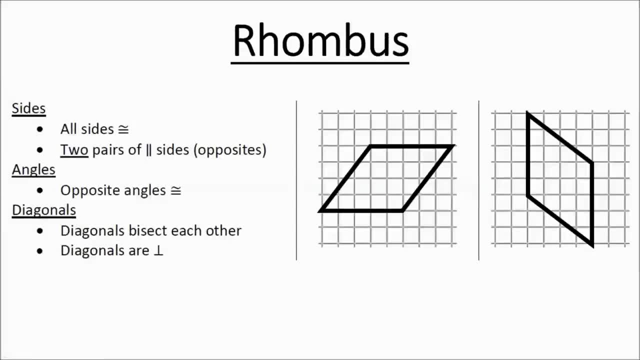 So that's the information for a square. If you want, you can do a screenshot of it. Good Moving on. So next is a rhombus. I've got two pictures of a rhombus. Regarding sides: all sides are congruent. 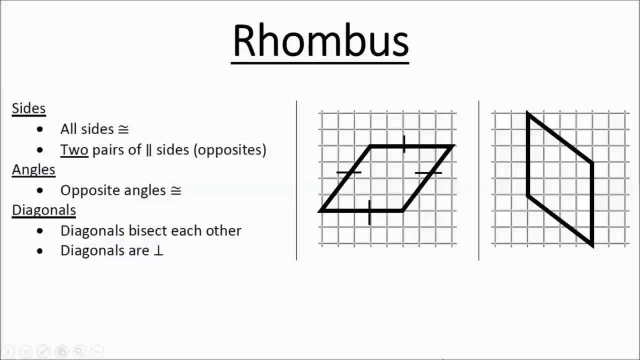 So we're going to put in some markers showing that they're all the same sides And then they also have two pairs of parallel sides, just like squares. So opposite sides are parallel- Two pairs of parallel sides. Regarding angles, opposite angles have the same measurement. 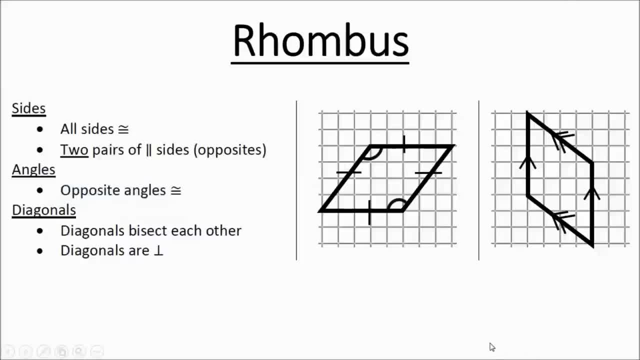 Opposite angles are congruent. So you'll see things like this: You'll see a single arc opposite a single arc, And then in these other corners you'll see a double arc and a double arc. That means their measurements would be the same. 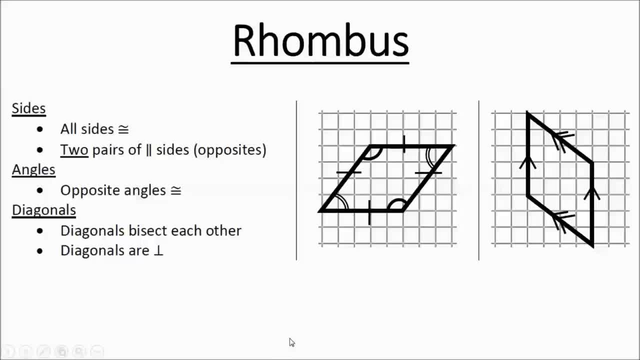 Those are the opposite angles, Diagonals. The diagonals are not going to be congruent, but they will cut each other in half, So they're going to bisect each other. So there's a diagonal, there's a diagonal. 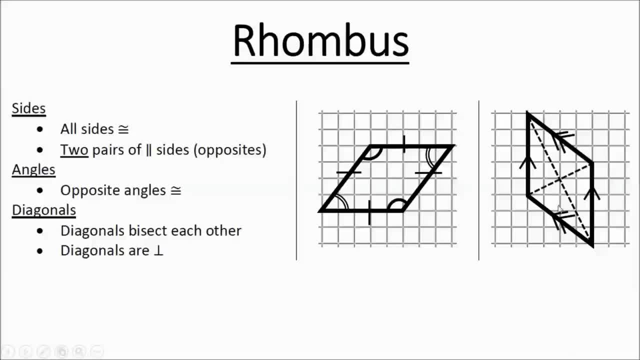 They're definitely not the same length, but they do cut each other in half. So you'll see these kinds of markings: This half is equal to this half, and then that smaller half and smaller half, And they are perpendicular. The diagonals are perpendicular, so sometimes you'll see a little square in there, signifying that they meet at 90 degrees. 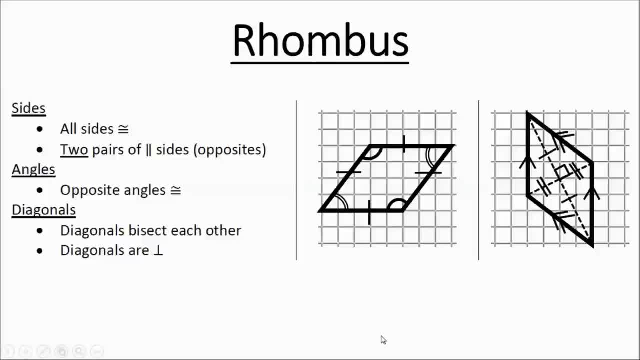 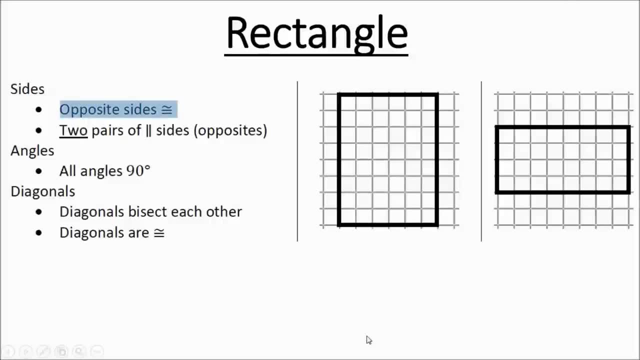 So that's a rhombus. Once again, you can screenshot that if you want Rectangles. So now we no longer have all sides being the same, but we have opposite sides having the same measurement. Opposite sides are congruent. 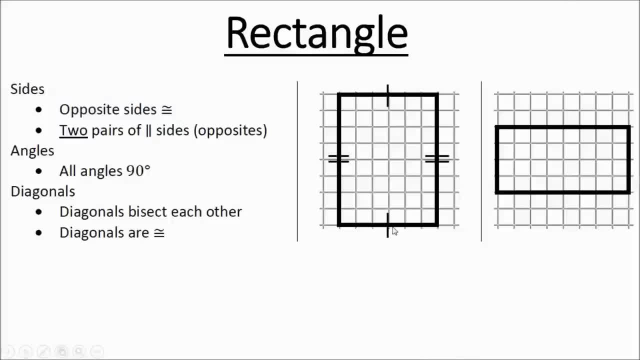 So you'll see marks like this: A single is congruent to a single slash, A double slash is congruent to a double slash. And for rectangles the opposite sides are congruent. So parallel sides, Two pairs of parallel sides. You'll see them marked like this: 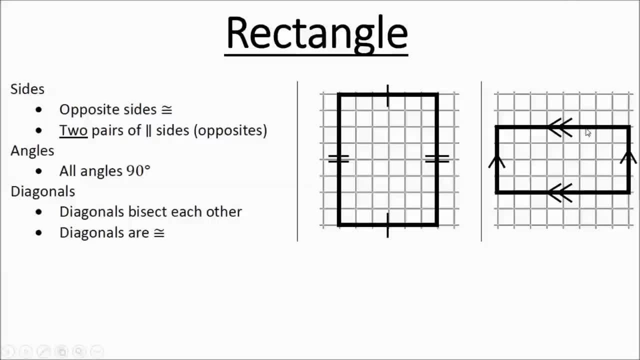 That means they're parallel, and double arrows also mean that these two are parallel. All angles are 90 degrees. That means four 90 degree angles. Now we're going to talk about diagonals. The diagonals bisect each other. They chop each other in half. 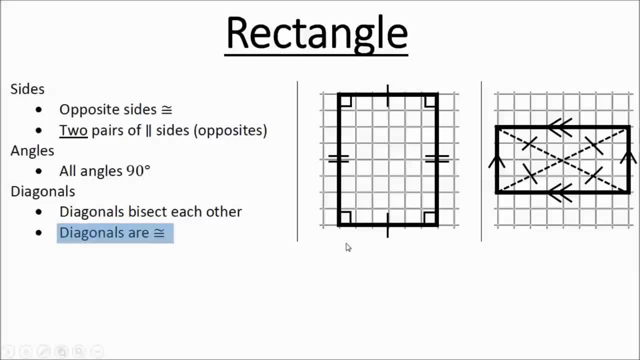 And they're exactly the same, They are congruent. So we have one diagonal, two diagonal and they cut each other in half. And there you go, That's rectangle. So this is another one you'd want to do a screenshot of. 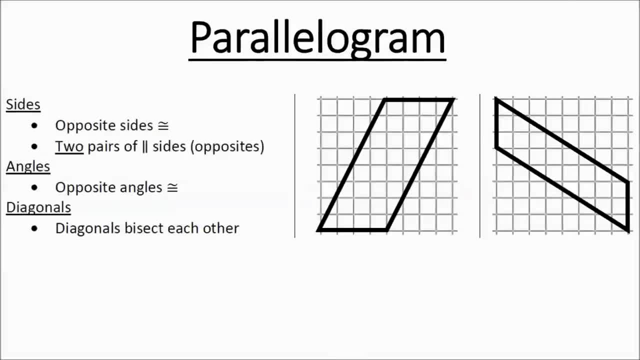 Next up is a parallelogram. Parallelogram has opposite sides, congruent. Opposite sides being congruent, you'd see these symbols: Two pairs of parallel sides. So here we've got double arrows and single arrows. The opposite sides are parallel. 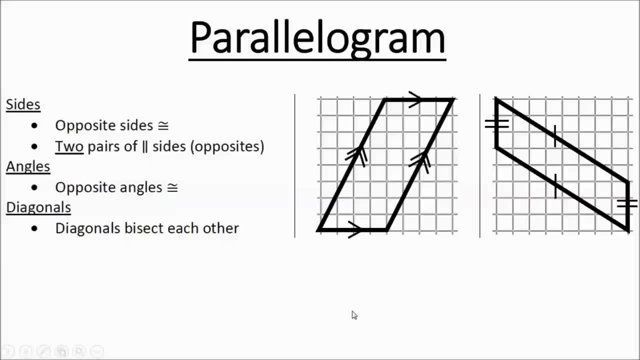 And opposite sides are congruent For angles. you've got the opposite angles being the same. Single arc to single arc, Double arc to double arc, And then diagonals. they bisect each other, They cut each other in half. There's nothing else you can really say about them. 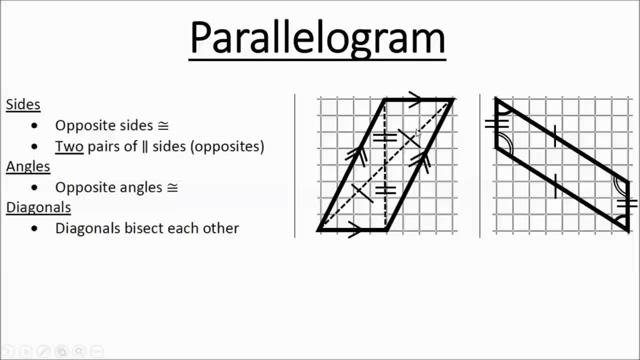 They do chop each other in half though, So this side's chopped in half, And then this double slash is the same as that double slash, But they're not perpendicular or anything like that, So that's a parallelogram. Next up is a trapezoid. 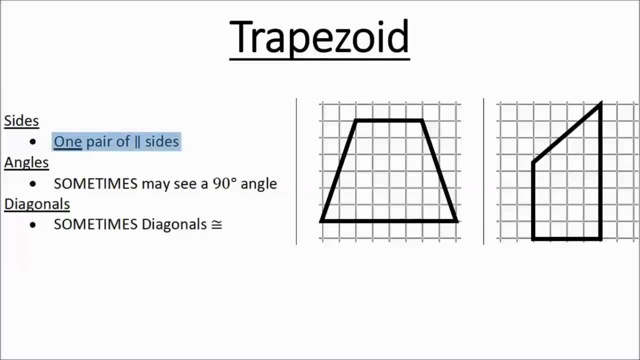 A trapezoid has only one pair of parallel sides, So this one on the left is usually the one kids are used to seeing. They see the two opposite sides being parallel. These other two sides are not going to be parallel Over here. this is the one that the kids usually don't remember or they don't realize. 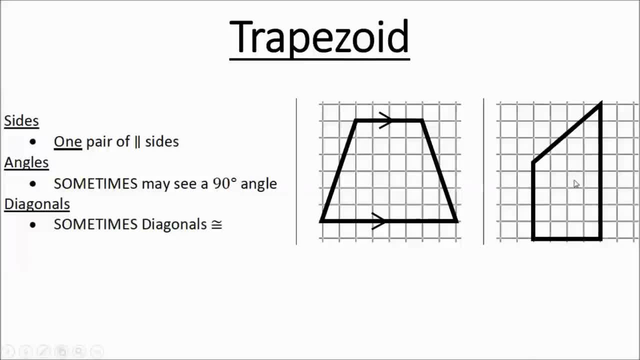 Because the top and bottom sides aren't parallel, but the vertical sides are parallel to each other. They would stay the same distance apart. Sometimes you might see some 90 degree angles, but it's not a rule. It's not like you have to have 90 degree angles. 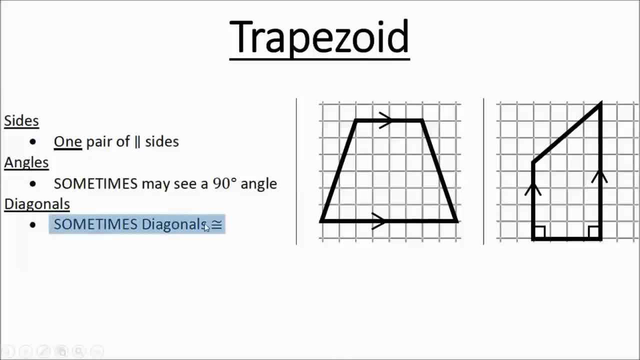 Sometimes it might happen. Sometimes you'll have diagonals be congruent, And that's fine, But it's not a rule. The only thing that's definite is the very first thing regarding the sides: One pair of parallel sides. You can do a screenshot of that if you want. 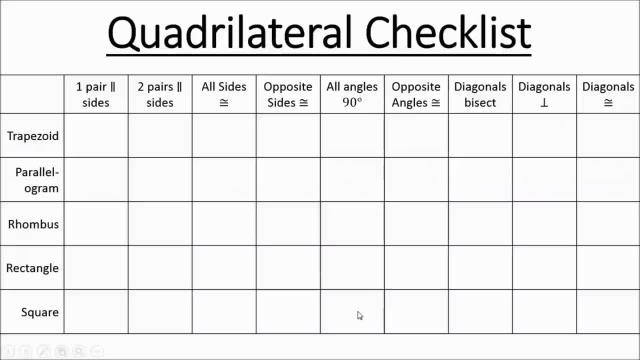 Alright, moving on. So now we're going to do a checklist. We're going to look at each shape and talk about all these different attributes. So one pair of parallel sides. The only figure over here that has one pair of parallel sides is going to be the trapezoid. 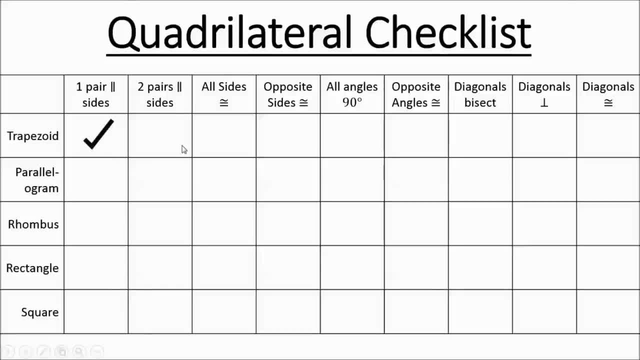 Regarding two pairs of parallel sides. All the rest of these have two pairs of parallel sides, All sides being congruent. There are only two of these quadrilaterals that have all sides congruent, And that's going to be the rhombus and the square. 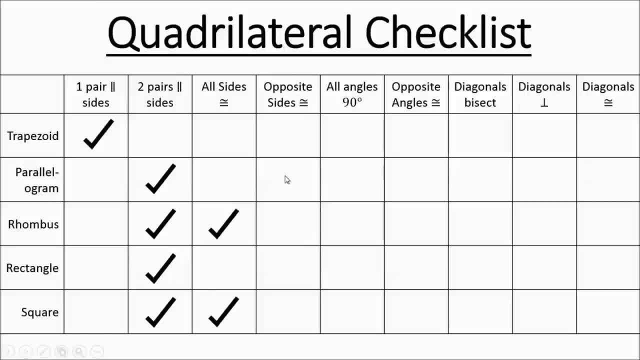 Regarding opposite sides, All of these, except the trapezoids, are going to have opposite sides being congruent, All angles being 90 degrees. The only two that are going to always have 90 degrees Are the rectangle and square, Opposite angles being congruent. 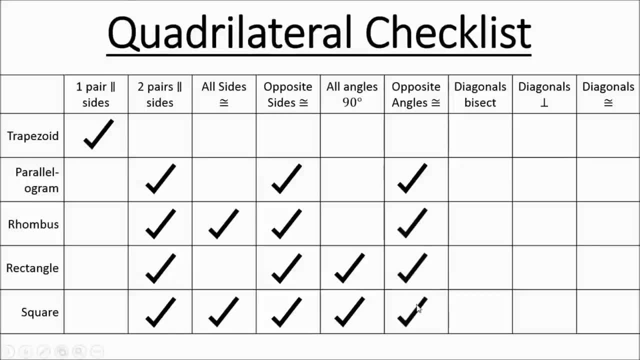 Is going to be everything except trapezoid. Now, with rectangle and square, Those opposite angles are congruent and they're 90 degrees, But they're still opposite and the same Diagonals bisecting each other. This is where it starts to get complicated. 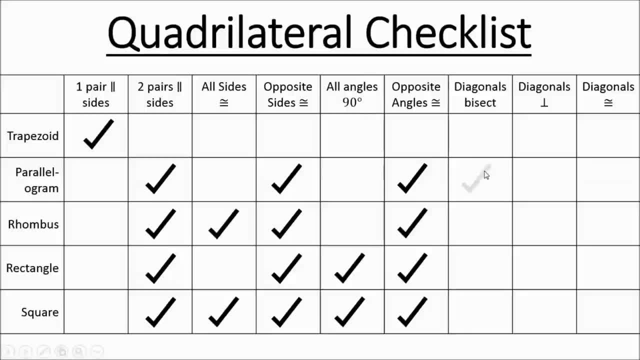 Diagonals bisecting each other is going to work for parallelogram: rhombus, rectangle and square. All four of those diagonals chop each other in half when they intersect. Now are diagonals perpendicular Only for the rhombus and square. 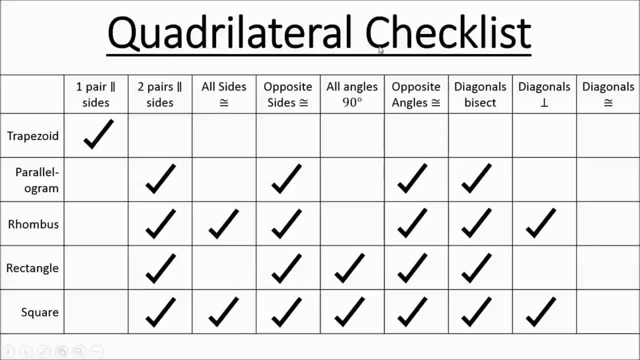 So when all the sides are the same, The diagonals are perpendicular. When the diagonals are congruent, That's only going to be for rectangle and square, For rectangle and square. That's when The diagonals are congruent. Finally, we're going to show one more thing. 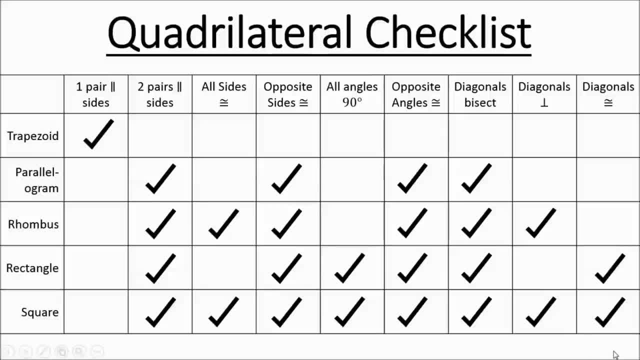 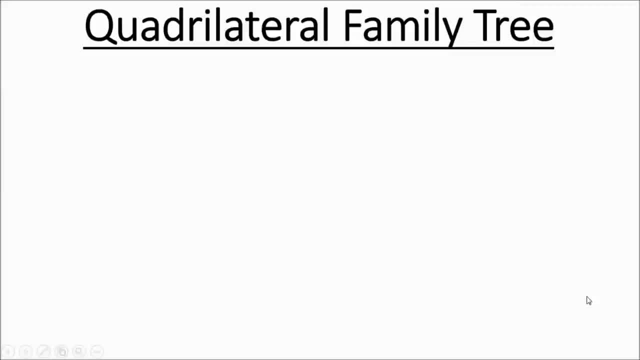 You can do a screenshot of this if you want. And we're going to show one more thing: Quadrilateral family tree. This is just another way to think about things. We're going to list the quadrilaterals at the top. This is anything with four sides. 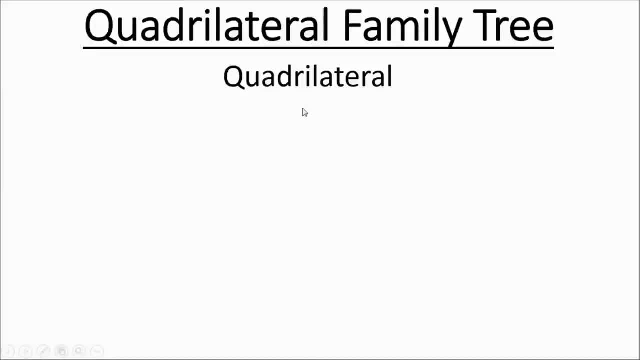 We're focusing on the parallel sides, But there are some quadrilaterals that don't have any pairs of parallel sides. We're only focusing on parallel, So we have our trapezoid, which was one pair of parallel sides. There's no other subgroups coming off of that. 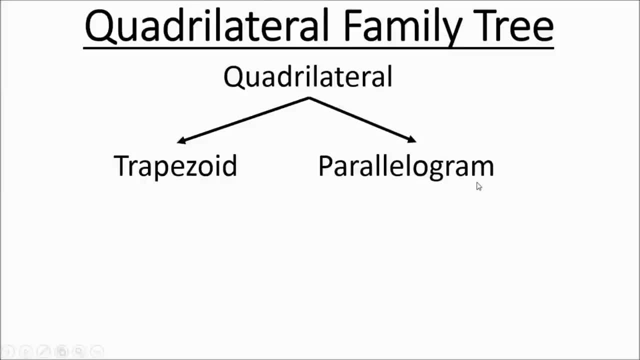 But over here we're going to have the parallelogram, So that's two pairs of parallel sides Of parallelograms. you can break them into two groups: One group having 90 degree angles, Parallelograms with 90 degree angles. 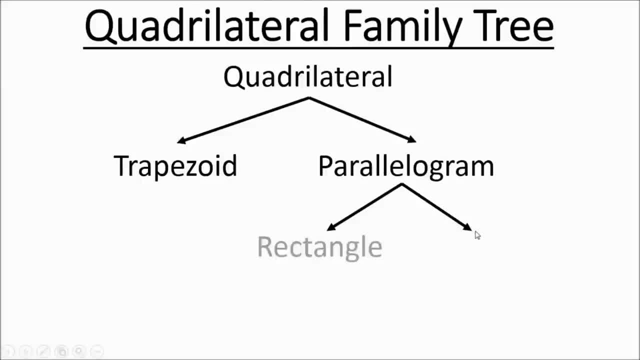 And parallelograms with all sides the same. That would be rectangle and rhombus, And then from here they kind of merge back together, Because if you take a parallelogram that has 90 degrees and all sides the same, You're going to get a square. 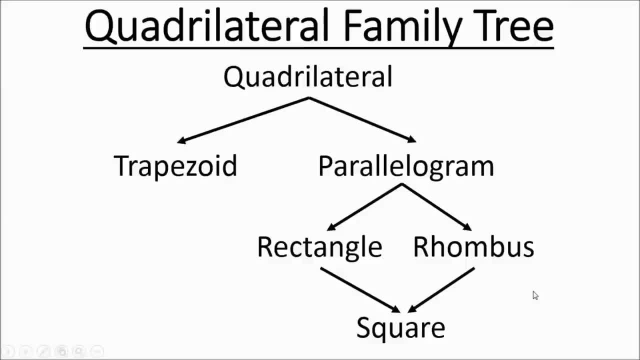 Now there's going to be some questions you might see on a test Where they might ask: is a square always a parallelogram, Or is a parallelogram always a square? And the way you want to figure this out is which one's underneath? 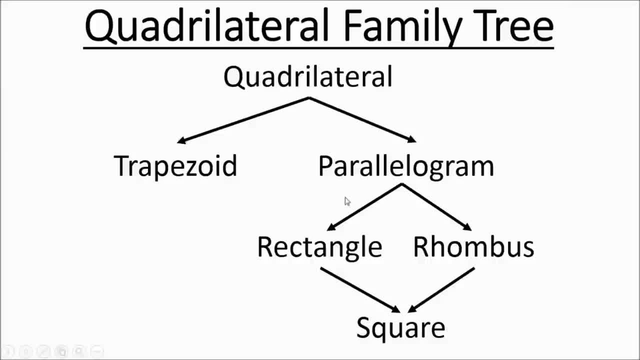 If it's underneath the other name, that means it is going to be part of that group. But if it's above the name, Or if it's not even in the same branches, It's not going to be part of that group. So you could say that a square is always going to be considered a parallelogram. 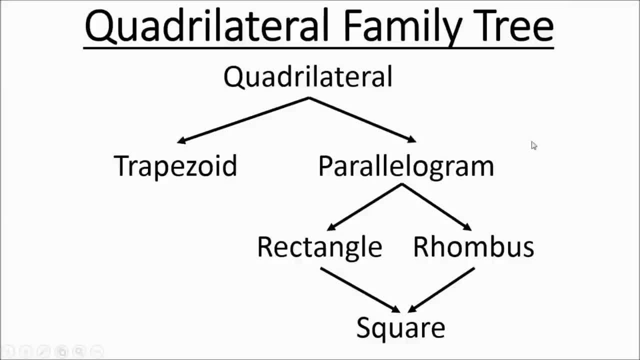 But you can't say that a parallelogram is always going to be a square. Or is a trapezoid always going to be a square? No, it would never be a square. Is a trapezoid always going to be a quadrilateral? 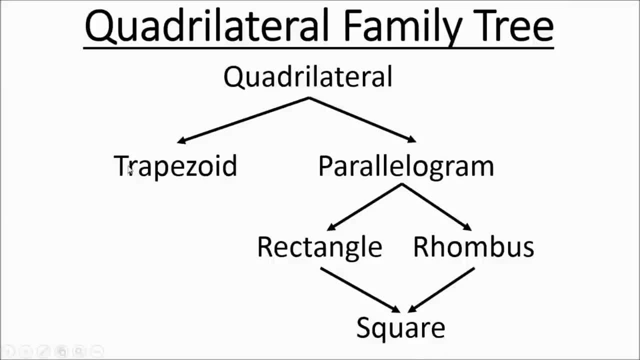 Yes, Is a square going to be a trapezoid? No, And this is because you put it on top of the same family tree, So you'll probably practice this more with your teacher in class. This is just another thing you might want to get a screenshot of. 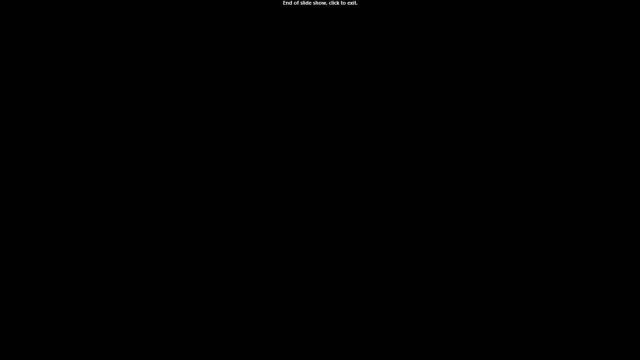 That's about it. I hope this helps. Best of luck to you. Bye, Excellent.